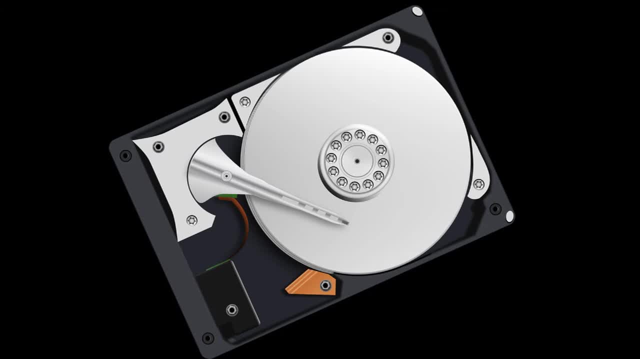 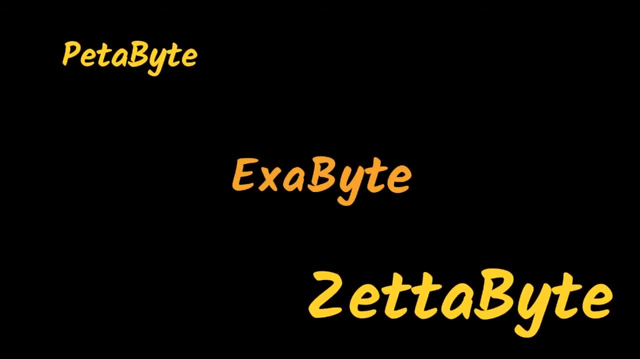 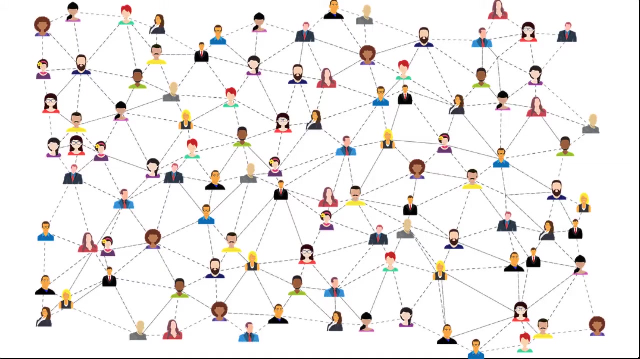 buy a 2TB hard disk or maybe two pieces of 2TB hard disk and put it inside a computer, but when you go to petabyte, exabyte and zettabyte, then a single computer completely fails to store all that information. and this has become very, very important because of the internet boom. 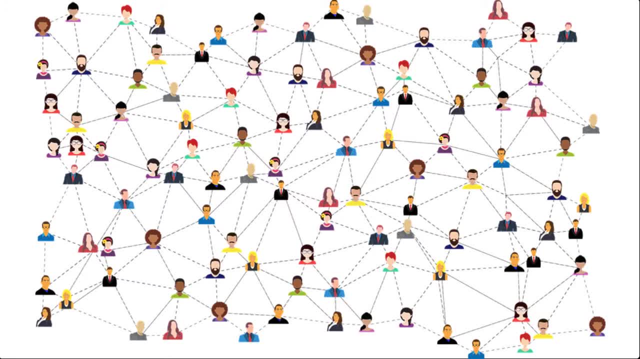 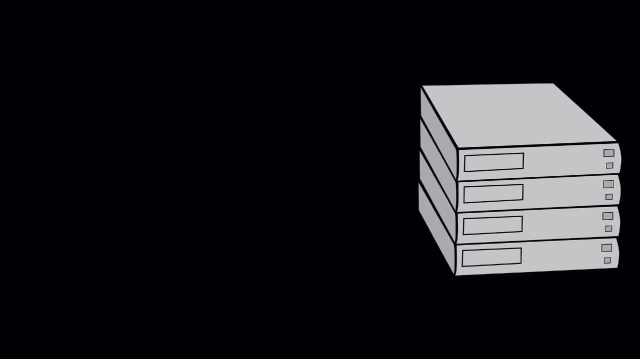 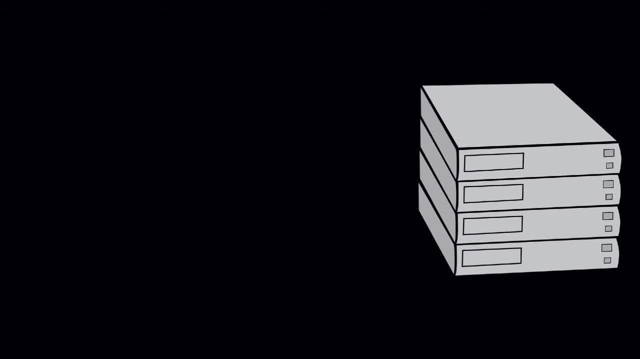 been in use since ever, and there is also concept of parallel programming, which can be implemented using techniques like MPI. So then, what's special about big data? you know, you can always use those traditional techniques of you know, clustering and parallel programming to address this problem. 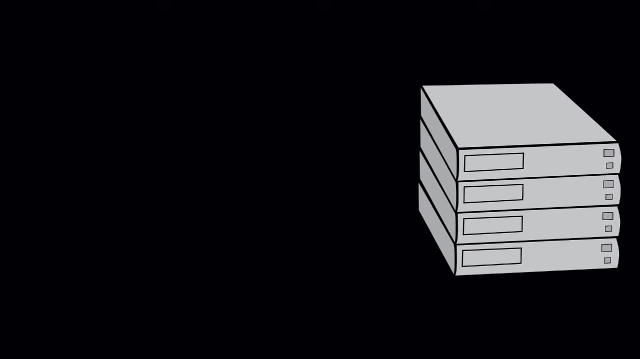 As it turns out, the main problem with that kind of an approach is that in your parallel programming the entire program with the division of the task to various nodes in your cluster has to be done by the programmer by hand. and that can be very, very taxing, especially because the 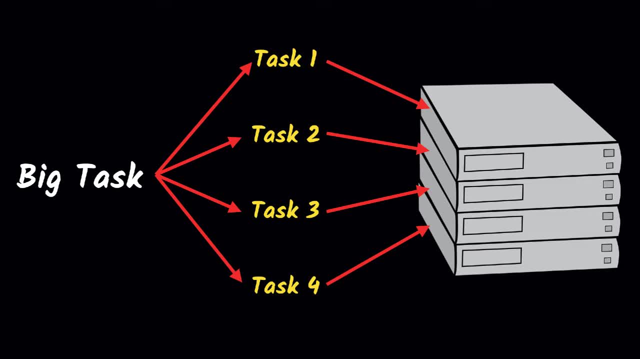 variety of data that comes into the big data machines is very, very wide. you know, if you had only one kind of data coming in at a particular rate, then still you could hire a software programmer to write a code that works for your system. But there is still a lot of data coming in at a particular rate and that can be very, very taxing. 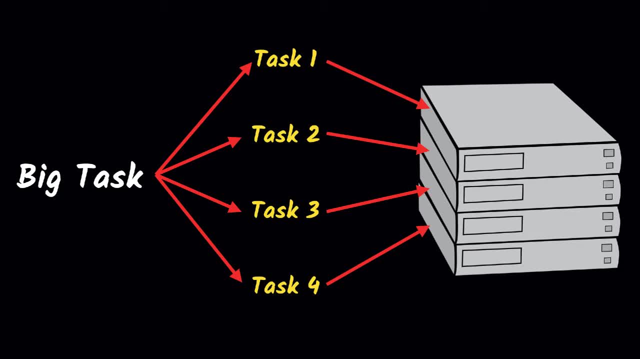 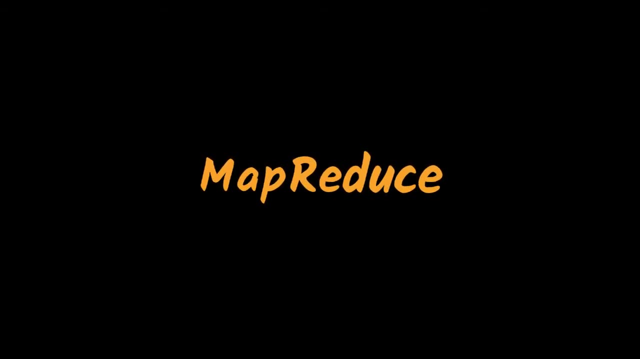 So there is so much variety in today's internet space that a standardized approach does not really work. and to handle this problem, Google came up with this algorithm called MapReduce, which not only did this segregation of your incoming data and processing into different chunks, but it also incorporated algorithms to do optimization and load balancing so that the 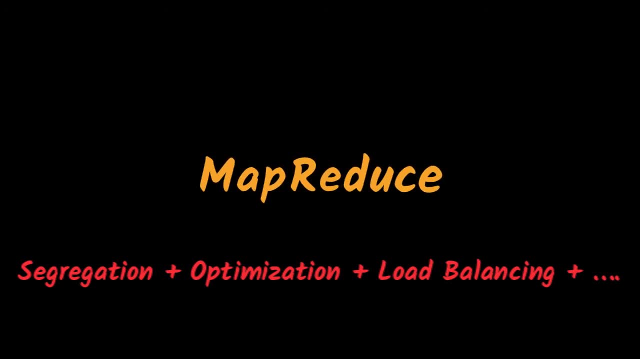 individual software programmer can do the optimization and load balancing. And that transition from conventional clusters and parallel programming to the use of these sophisticated algorithms like MapReduce is what is the leap that computer science has made over the past decade or so. So essentially, big data requires a set of techniques and technologies with new forms of 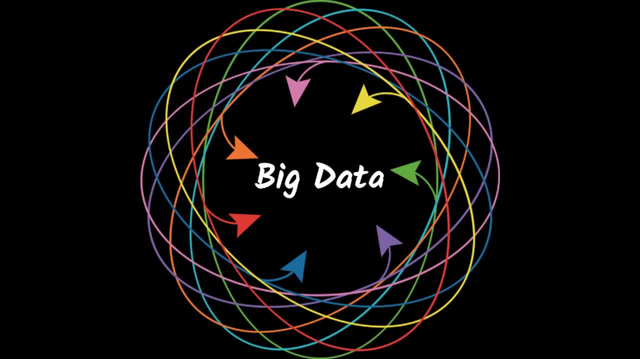 integration to reveal insights from data sets that are diverse, complex and of a massive scale. You know massive means we not only are limited to petabyte, but are now even moving to exabyte and zettabyte. Now, big data has a lot of characteristics which are important to take into consideration. 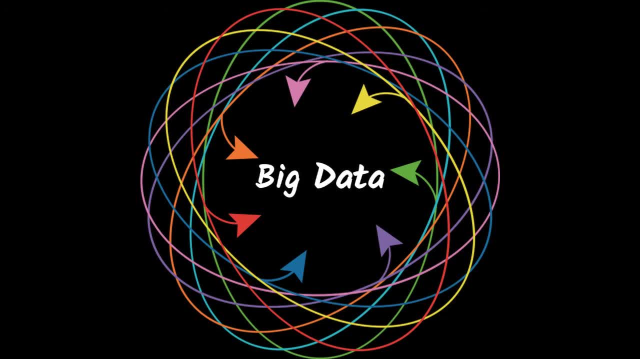 in order to design a good big data algorithm, and that list is very, very long, but we are going to discuss some of the most important characteristics of big data that you need to keep in mind. So these are the six V's: the six V's of big data. 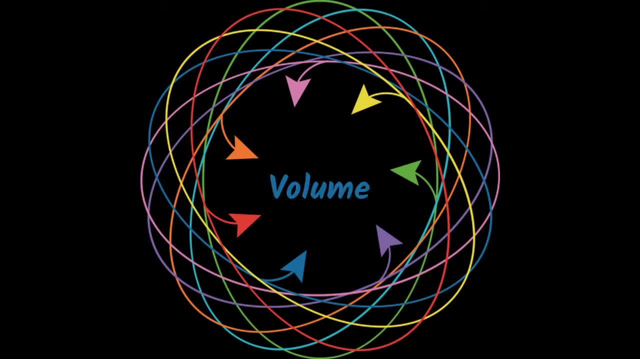 The first V is volume and it refers to the quantity of the generated and stored data. As I just mentioned, big data deals with, you know, exabytes and zettabytes of data, which is an enormous amount of data volume. So your big data technology has to be able to handle this amount of volume. 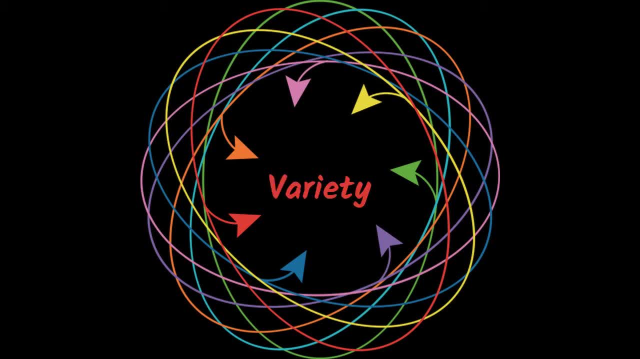 The second V is variety. As I just said that You know, in the standard paddle processing algorithms or clusters, in the early 2000s or before that you had one kind of data coming into your algorithm. but because of this internet boom, now your same piece of software has to handle structured, semi structured as well. 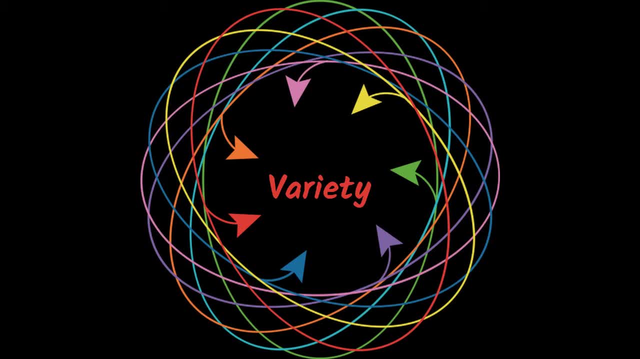 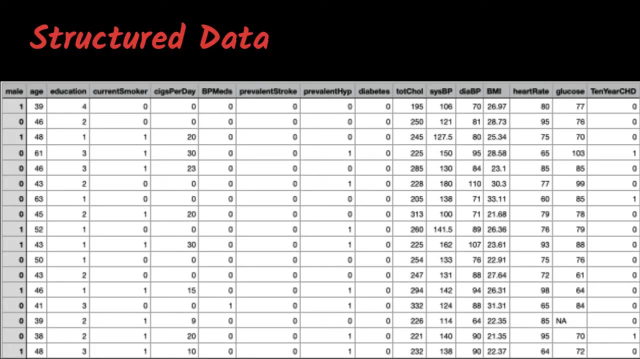 as unstructured data in the form of text, images, audio as well as video, And these are captured through various sources like social network, internet browsing, log files, Sensors and devices like this. structured data is something that is present in the form of data tables. You know, for example, if you take an excel sheet, that is an example of structured data. 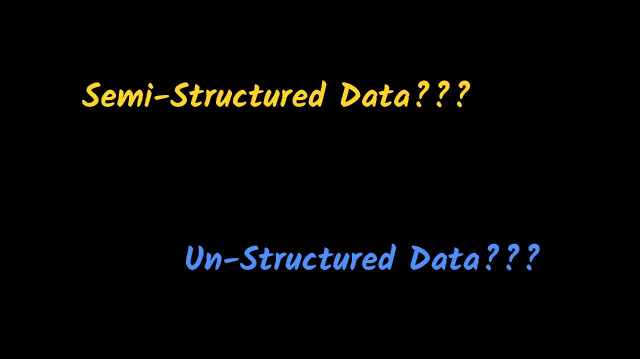 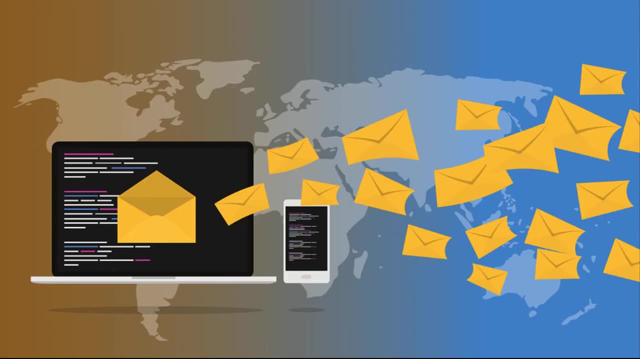 which is very well known to us. semi structured data and unstructured data are relatively not very familiar terms, But if you take email, you know which is something that all of us are familiar with. that is an example of semi structured data. What is it? 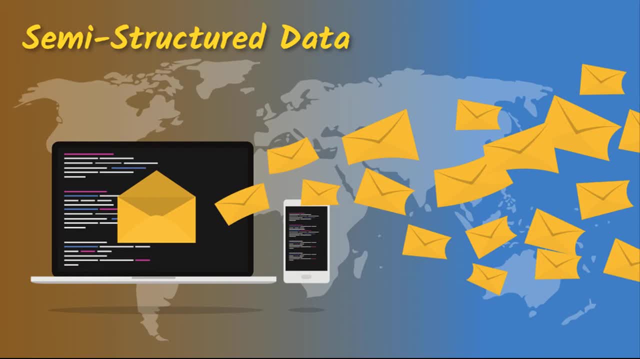 Why is it semi structured? Because it contains structured components like name, email address, recipient, date of the email, time of the email and so on, And it can also be organized into various folders like the inbox and, you know, sent trash, etc. So that gives a structure to your email. 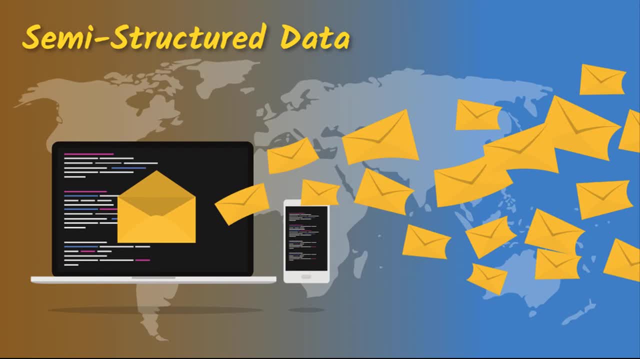 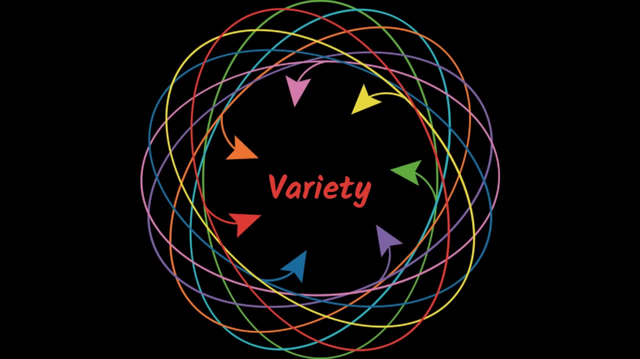 However, the email also contains the text of the email, the main body of the email, which is unstructured data, Because you cannot organize that in a simple tabular form. So this is the kind of variety that your big data technology has to deal with, and this 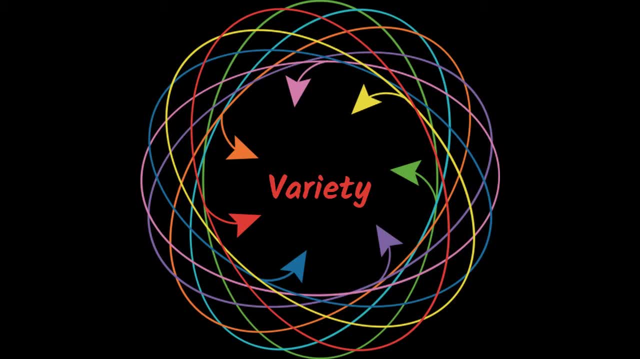 is the second V of the big data characteristic. The third V of big data is velocity, and this is the speed at which data is generated and processed. In current times, where even a millisecond is a long time, you need algorithms that can process this. 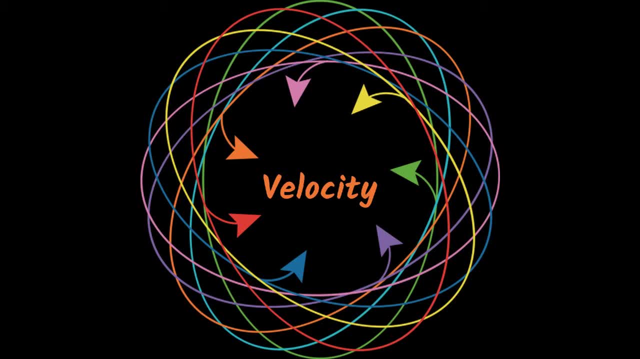 The fourth V of big data is massive amount of data in a relatively very, very short amount of time, And this calls for massive amounts of optimization, which algorithms like MapReduce are excellent at. The fourth V of big data is veracity, which refers to the truthfulness or reliability 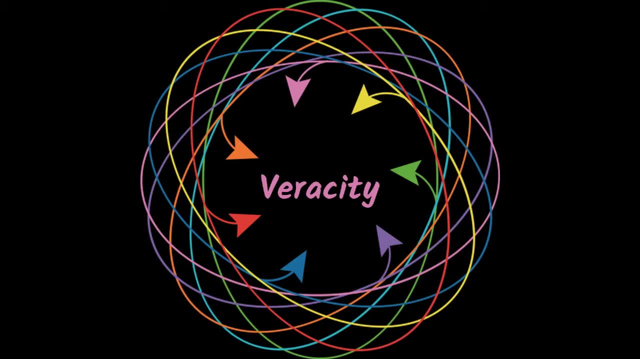 of the data. You know you may get data in, you know exabytes and zettabytes and you may be able to store it. But if the storage is not of good quality, Then you are into trouble. So, for example, when you get data from all these different streams and you send them. 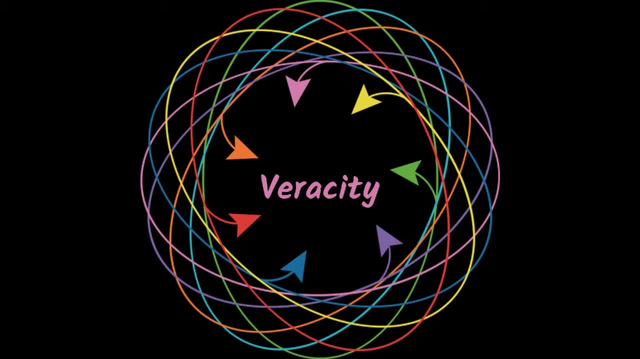 to clusters. There has to be some redundancy built in so that even if one of the cluster goes down, you still can access that data from another cluster. So you need to make sure that the data which is stored is truthful as well as reliable, So that even when you access that after a year or two years, you know that there is no. 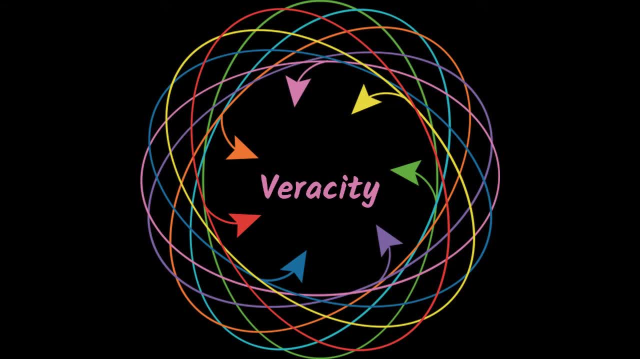 corruption which has happened. And this is the fourth V of big data. The fifth V of big data is value, which means that what is the worth in information that can be achieved by processing and analyzing of large data sets- You know you don't want to store this- exabytes and zettabytes of data for nothing. 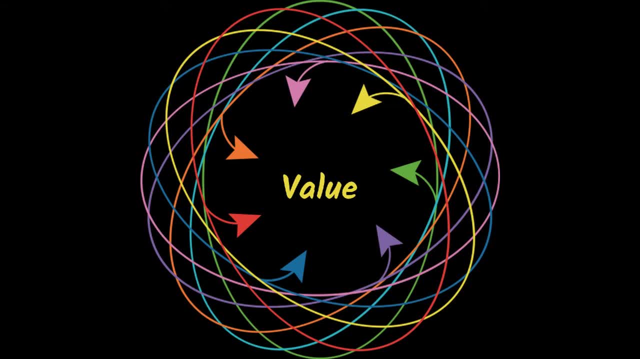 You finally want to analyze them in order to get insights which can lead to development of your business, And that is why, When implementing any particular big data technology, You also have to think of the value, which means what is its processing ability, so that you can get the required information for your business needs. 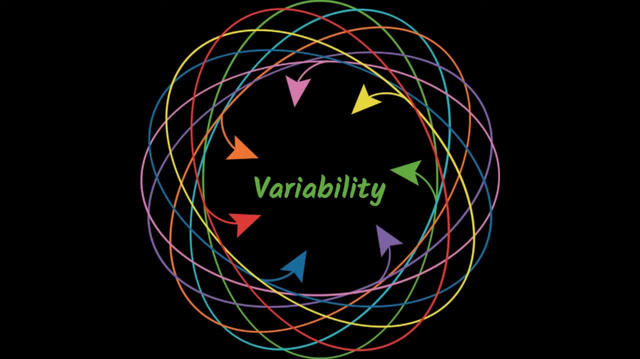 And the final V, or the sixth V, is variability, which means that is your big data technology something very, very rigid or is it flexible to be able to handle the changing formats, structure and sources of big data? You know This space is changing so fast that something which is in fashion today may go out of fashion. 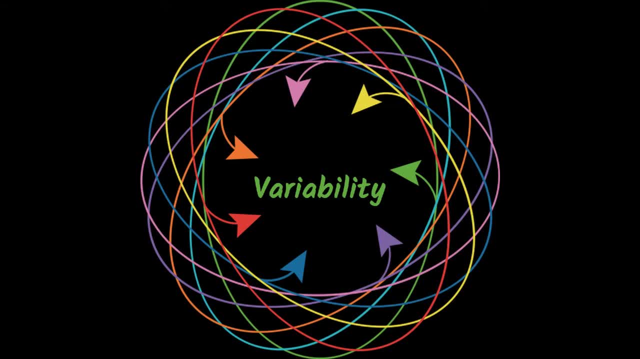 six months from now. So your big data technology has to be variable enough to be able to handle these changes. You know you don't want to completely have a new system installed every six months. You want to have a system that works over a longer period of time. 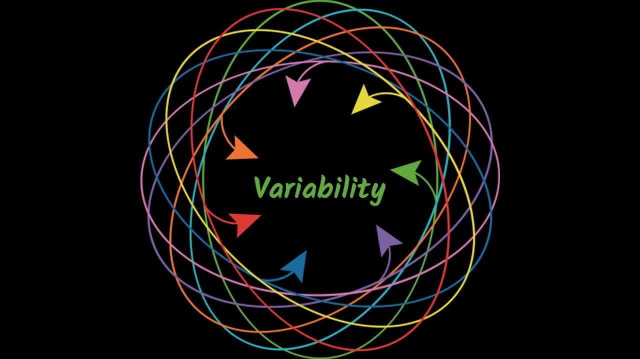 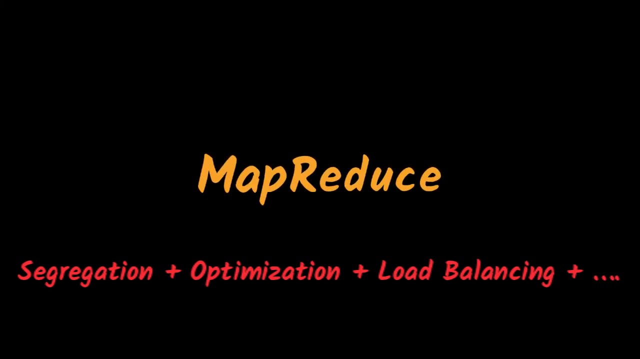 And so your big data technology also needs to incorporate this notion of variability in order to take care of these changing formats, Structure and sources of big data. So, as I mentioned, one of the fundamental advances in this field was made by Google in the form of MapReduce algorithm, which has kind of become the bedrock of all the major big data technologies. 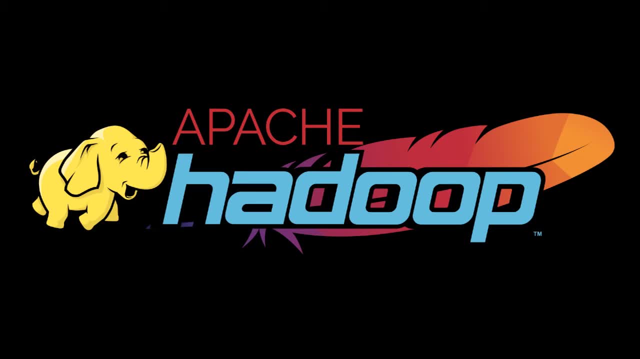 and Apache. Hadoop, which is the most popular open source framework today for big data, is based on this MapReduce algorithm, and this MapReduce, of course, does parallel processing, which means it breaks your incoming data and processing requirements into various chunks. But, as I mentioned, that can be done even by traditional parallel processing algorithms. 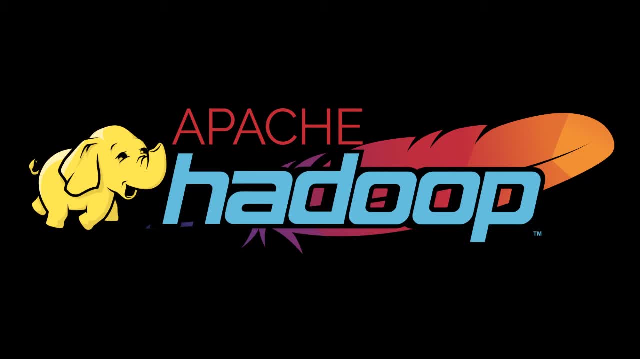 like MPI. So where MapReduce comes in, and why is it so magical, is that it does all the segregation, optimization and load balancing on its own, without the user having to specify that explicitly, And that is why it becomes so easy to use these big data technologies. 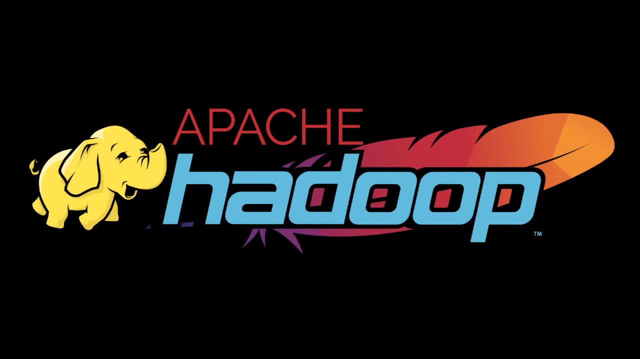 Because dividing a given piece of work into chunks is not really a big deal. It is the optimization, and how you actually send this to different clusters in order to maximize the processing and storage speed is what really matters, and this is what the MapReduce algorithm takes care for you. 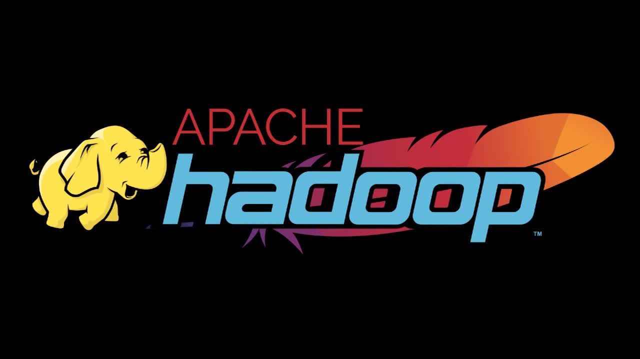 So Apache Hadoop is an open source framework that allows you to store and process big data in a distributed environment across clusters of computers using very simple and easy to use programming models, And currently Apache Hadoop is, like you know, almost a default choice for big data algorithms. and one of the biggest Apache Hadoop servers is the Yahoo cluster which has, you know, thousands of CPUs running in a distributed fashion and has over more than 4000 nodes, And this is one of the biggest Apache Hadoop clusters in the planet as of now. 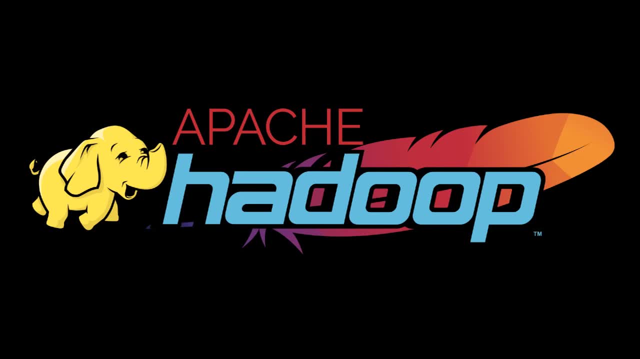 So the Apache Hadoop has mainly four components. The first is the Hadoop distribution. Hadoop is a distributed file system, or called HDFS. So this is the basic file system over which all other functions of Hadoop run. What it does is that it breaks down the data into small packets called blocks, and these 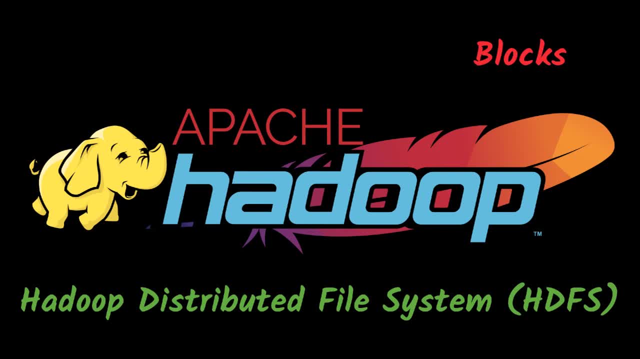 blocks are stored in a distributed manner and, to ensure some redundancy and to ensure that data is never really lost, it stores multiple copies of each block so as to prevent data loss due to server breakdown. Now these blocks of the Hadoop cluster can be of different sizes, but the typical size 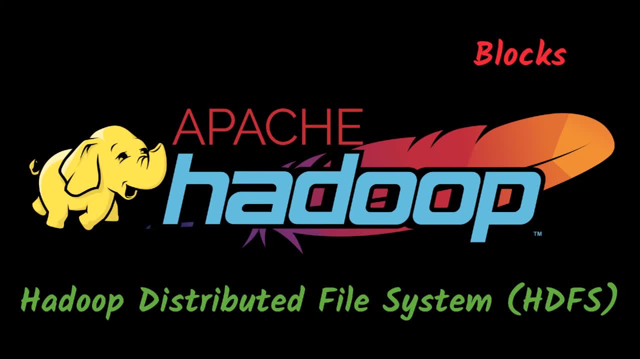 of each block currently is around 128 MB, And the reason it works so well is that computation is done at the data node itself. So wherever the data is stored, the Hadoop cluster or the Hadoop algorithm does the processing of the data there itself, so that there is less amount of back and forth between the 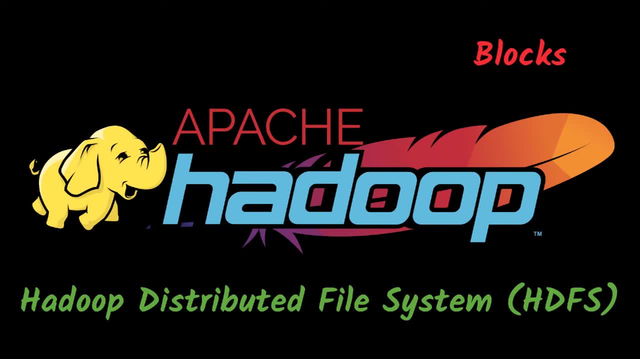 main node and the data node, And this is the Hadoop cluster. This helps in maximizing the efficiency of your big data technology. The second component of Hadoop is the MapReduce algorithm, which I have already mentioned to you earlier. So this is for parallel processing of each data block at the cluster node, and this was 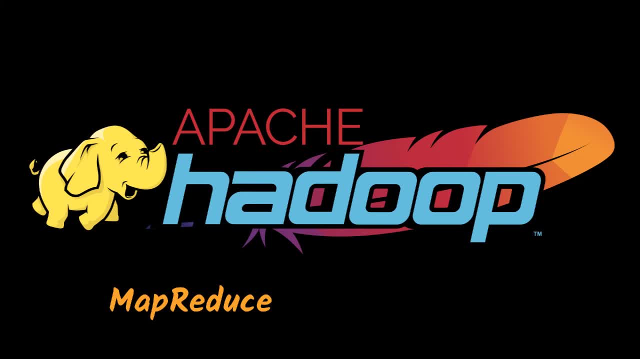 developed by scientists from Google. What it does is that it divides the task into small parts, assigns them to different computers and then collects the results to form an integrated output. And the best thing about this is that Hadoop is not just a database. 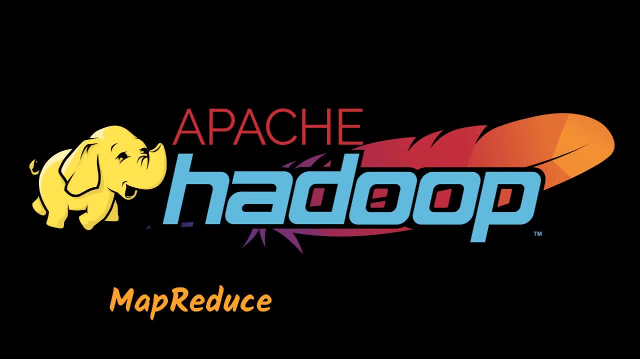 Hadoop is not just a database. Hadoop is not just a database, It is also a process map reduce, And the reason why it is so popular is that it automatically manages other aspects of the parallel processing framework, like process distribution, optimization and load balancing. 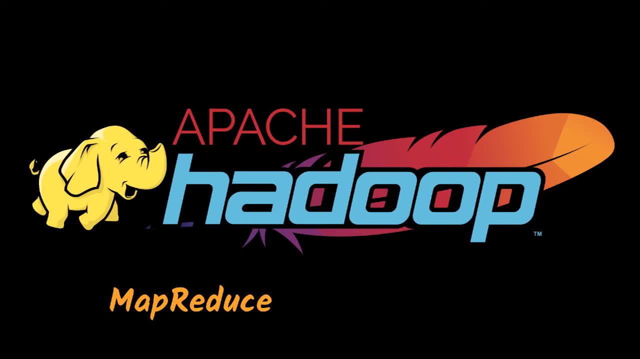 without the particular user or software programmer having to worry about all these details. So the map reduce, as you know, has two stages: map and reduce. The map or the mappers job is to process the input data, so the incoming file is in the form of a file or directory. 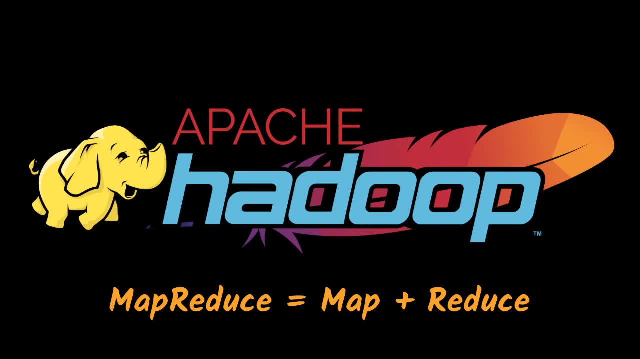 tree which is stored in the Hadoop distributed file system, HDFS, and then the input file is passed on to the mapper function, line by line. The mapper processes the data and creates several small chunks of data called blocks, and then you come to the reduce stage. So what this reduce? 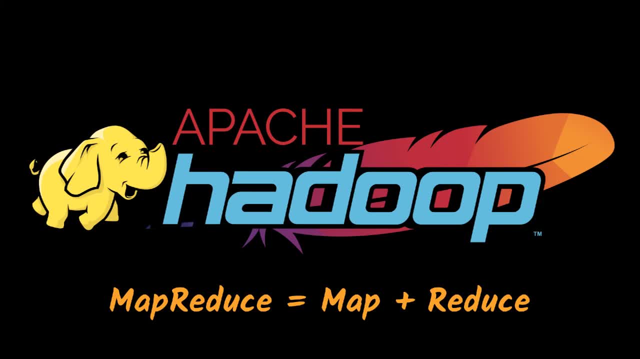 does is that it processes the data which is coming from the mapper and then produces a final integrated output which is then again stored in the HDFS framework. The third component of the Hadoop framework is the Hadoop common. So Hadoop common is just a set of libraries which is used. 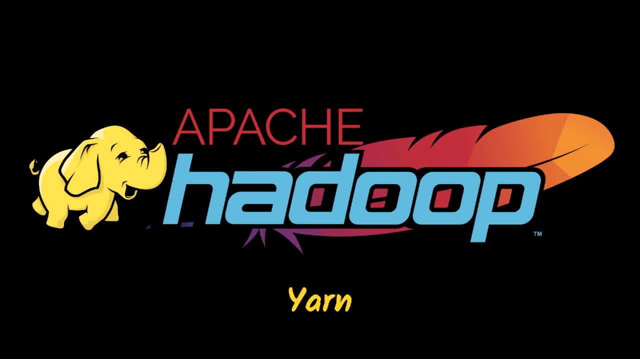 by the Hadoop framework. Then the fourth component is the Hadoop yarn. So this is a job scheduling and cluster management functionality of the Hadoop framework. So this Hadoop is excellent and it forms a bedrock for most of the big data technologies. currently, However, it is 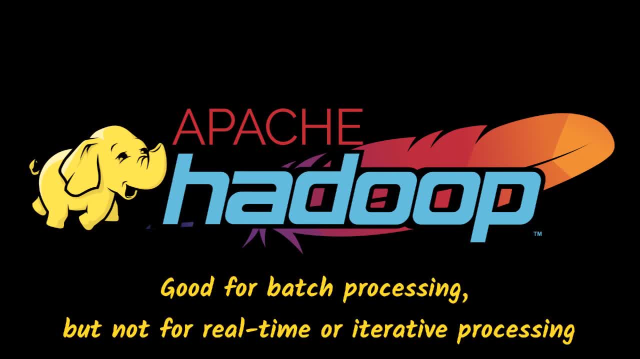 not very good for iterative algorithms like the k-means clustering, because the data has to be fetched from the hard disk multiple times and reading and writing from a hard disk multiple times is not very fast. And here comes another big data technology called Apache Spark which is built. 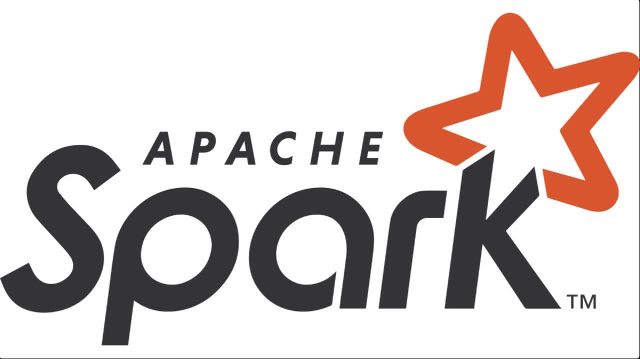 on top of the Hadoop MapReduce module and it extends the MapReduce model to efficiently use more type of compute. So this Hadoop is a very good example of the Hadoop app for using these applications which include iterative queries and stream processing. So because your Apache spark does the processing in the memory, 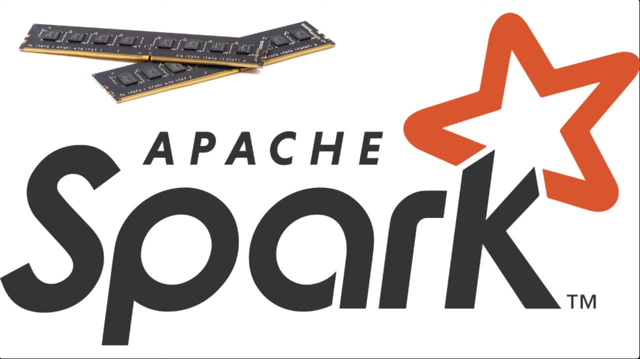 or the ram instead of the hard disk. it can run the application in Hadoop cluster many, many times faster than what the standard Hadoop framework. So this Apache spark uses Hadoop mainly for data storage functionality and it has its own cluster management and processing functions. 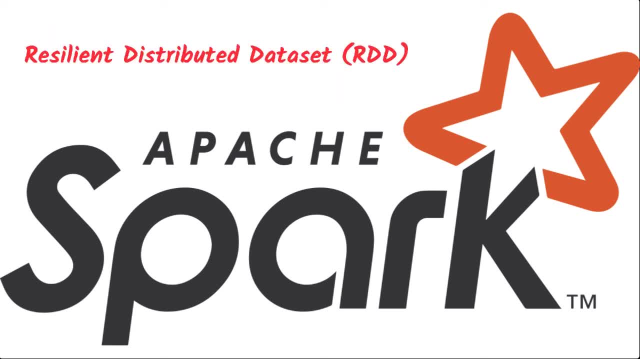 another framework called the Resilient Distributed Dataset or RDD, structure for processing the data, which makes it much, much faster. Apache Spark also has several built-in APIs in Java, Python or Scala which can make writing programs very, very easy in multiple manners. 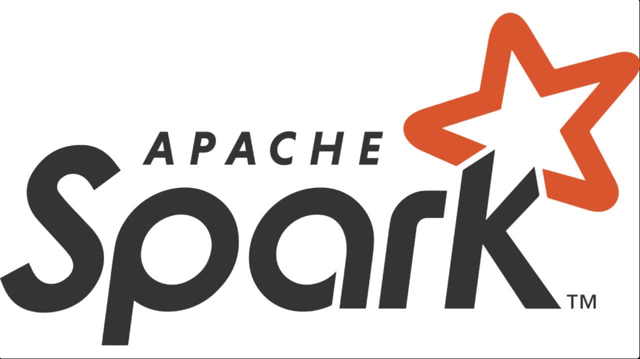 Apache Spark not only provides a map and reduce strategy, but also supports SQL queries, streaming data, machine learning and various kinds of other graph algorithms. So Hadoop is better for batch processing of data and Spark is better for real-time processing. And for real-time processing, Spark can be about 100 times faster than Hadoop.